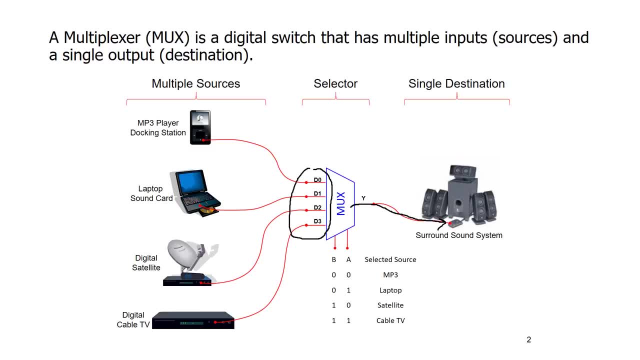 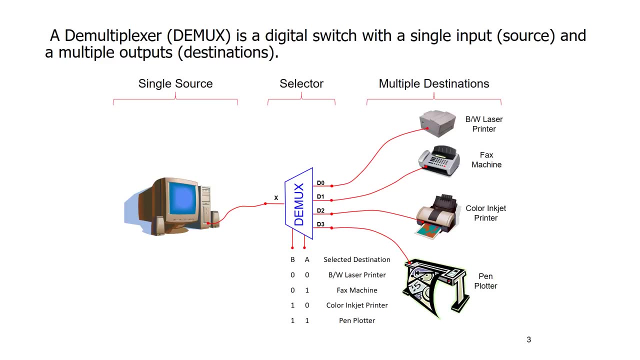 my speakers. So again, multiplexing or a multiplexer is several inputs, multiple inputs, a single output, and you can select which one of those inputs goes to that output. A demultiplexer, or demux as it's sometimes abbreviated, as is the opposite of a. 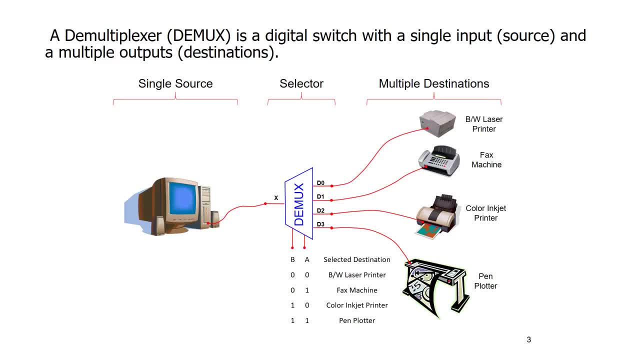 multiplexer, as you can see here. So a demultiplexer is a device that allows you to have multiple outputs. So I have one input. Here's my one input, this very old looking computer right here, my single input, and I have several output choices. So perhaps I have a document that. 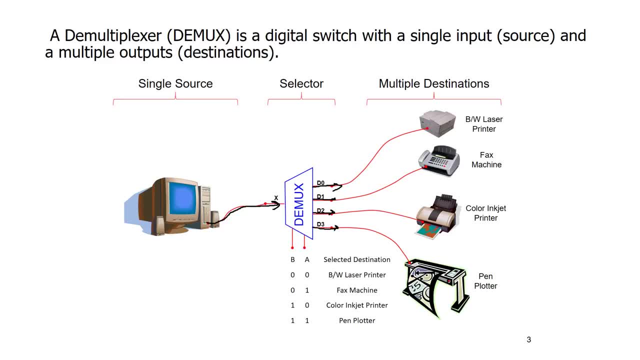 I want to print and I can select which of these outputs I want to send my document to. It might be my laser printer, my fax machine, my inkjet or a pen plot or so forth. So a demultiplexer. 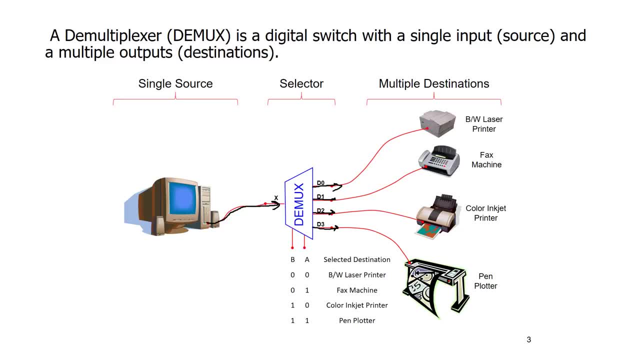 it's the opposite of a multiplexer. I have one input and multiple output And perhaps you noticed that the multiplexer, abbreviated MUX, was the same symbol as the demultiplexer, but it was the other way around, So my demultiplexer- they're both trapezoids One. 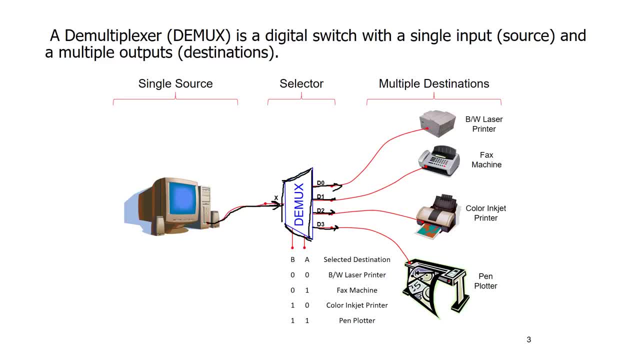 input, multiple outputs. that's my demultiplexer. My multiplexer was the exact opposite. in terms of its symbol. It looked like that right: It had multiple inputs, multiple inputs and a single output. That was my demultiplexer. So I had multiple inputs, multiple outputs and a single output. That was my demultiplexer. 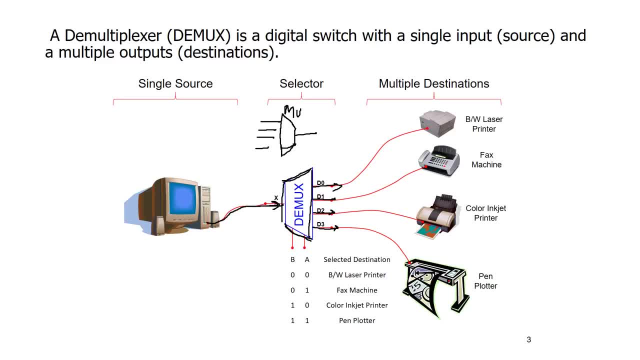 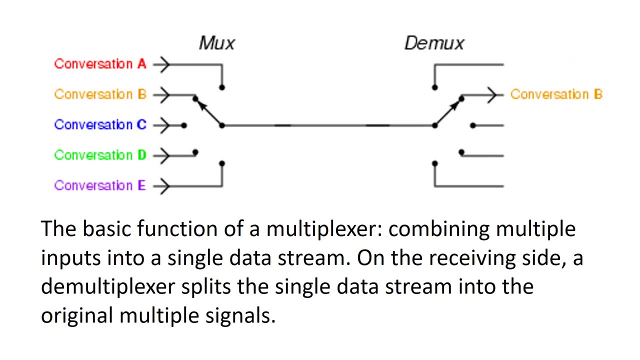 That was my multiplexer, abbreviated MUX. This is my demultiplexer: a single input, multiple outputs, And you can select where that output should go, where you have a bunch of different destinations, As you might have expected. multiplexers and demultiplexers. 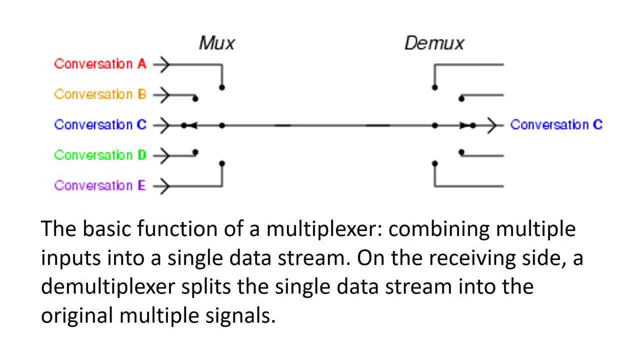 often work together. So here on the left I have a multiplexer showing multiple inputs combined into one output- Now, this output might be like a high-speed fiber optic cable or something like that- and on the other side I have a demultiplexer. 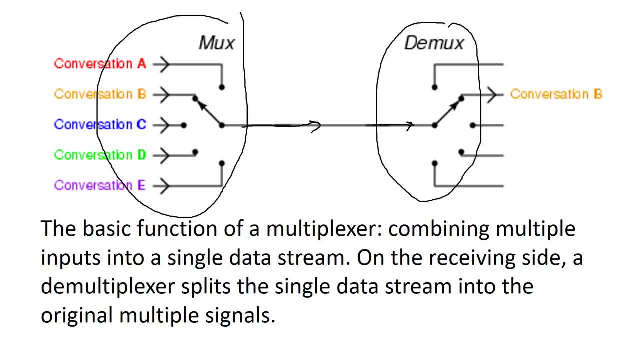 taking that single input and routing it to the correct output. So, multiplexer, multiple inputs- I have a bunch of inputs here. One output demultiplexer, that single input and it's sending it to the correct output. And in this illustration it shows that I have a bunch of conversations all happening at once. 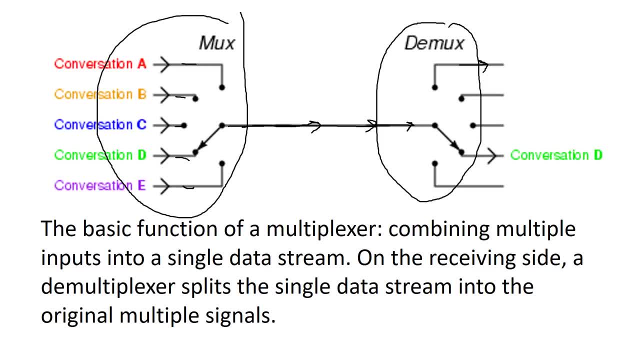 and these could be conversations between people or computers or whatever- and they're all getting combined into this single high-speed line and then it's getting routed to the correct recipient on the other end, using multiplexing to combine the inputs and demultiplexing to take the input and send it to the correct output. 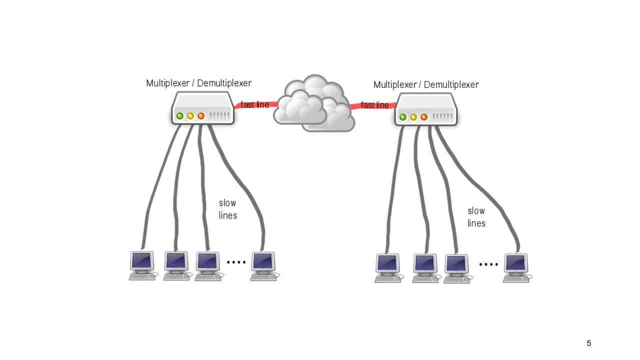 Here's another diagram showing a similar thing actually as the previous diagram, where I have a multiplexer Multiplexer. in this case it's called a multiplexer demultiplexer, because I might have several inputs. that's the multiplexing part. 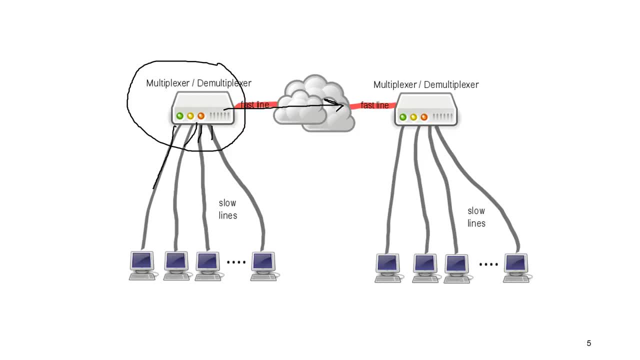 several inputs going to a single output, a fast line, as it says, and then getting demultiplexed, going to the correct output perhaps. so that's the demultiplexing part, but then on this side the communication might go the other direction as well. 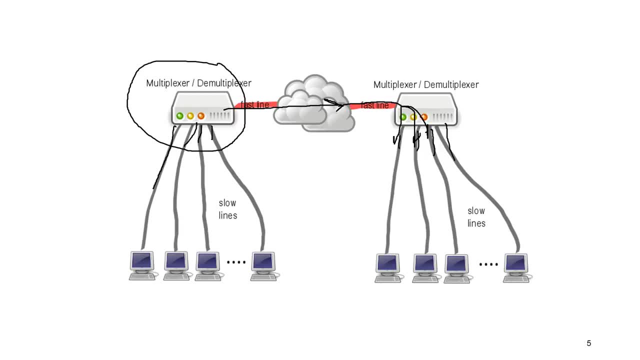 where I have several inputs. so this box is actually a multiplexer demultiplexer. here I might have several inputs going to my fast line and then again getting sent to my correct output. so depending on which way the communication is going, 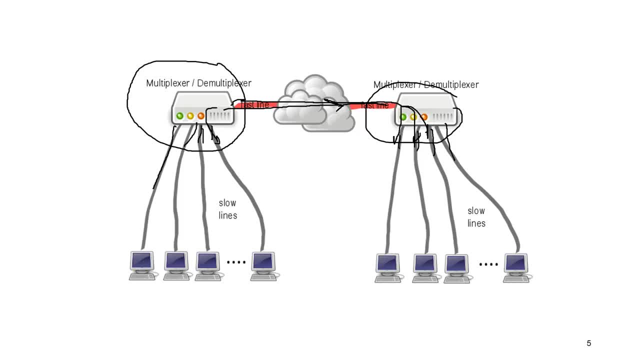 these boxes could either be multiplexing or demultiplexing, either combining several inputs to a single output or taking that single input and sending it to the correct output. I just thought this was a nice additional diagram to add. Now it's time to look inside a multiplexer. 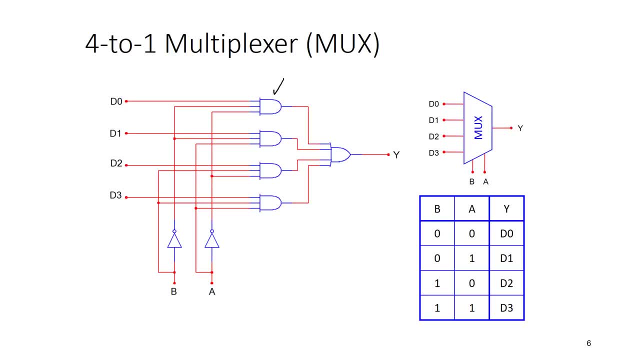 see how they work. A multiplexer is just built out of basic gates. Here's a 3-input AND gate, a 4-input OR gate. here's a couple of NOT gates, a couple of inverter gates, and let's see what's going on inside here. 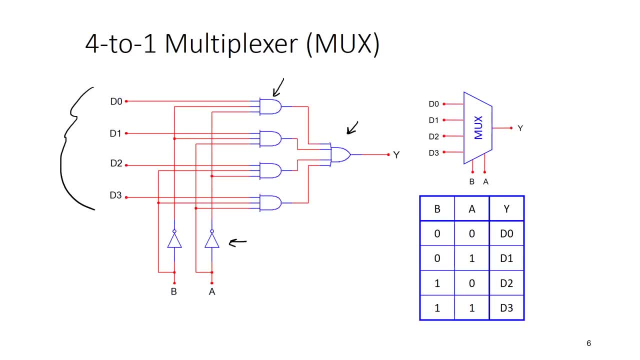 So this is a 4-to-1 multiplexer. I have four inputs. The number of inputs is always going to be some power of 2.. It's always going to be 2 to the N. In this case it's 2 squared. 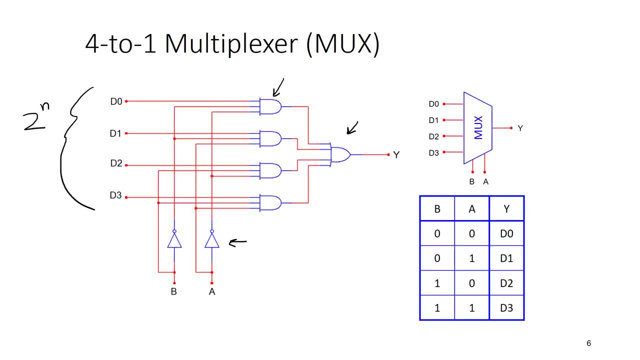 It's 2 squared is 4, but it could be 4 inputs 8, inputs 16, and so forth, and on the bottom here this is how I select which of these inputs goes to the output. So just real quick, before we get into how this works. 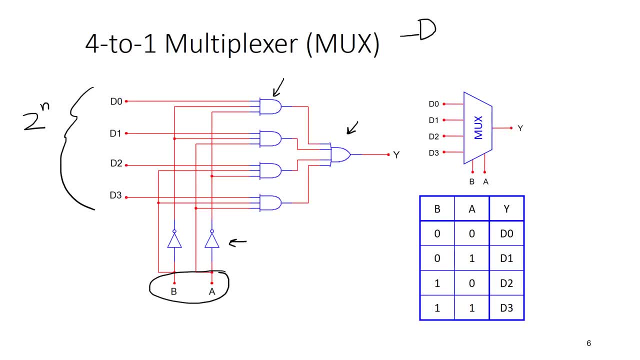 just to jog your memory about how AND gates work. if I send in a 0 to an AND gate, that output is always going to be 0, no matter what the input is. So let's say I have a switch here called A. 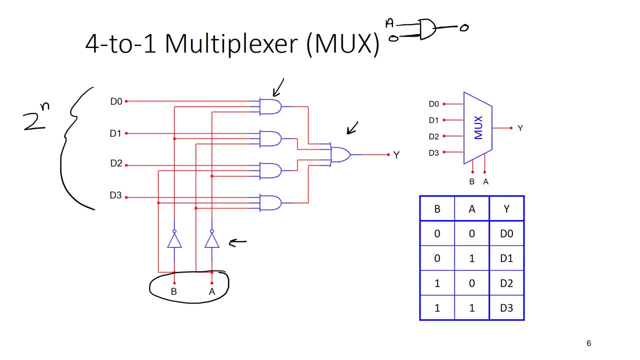 If I send in a 0 to the other input, the output's always going to be 0. So if you send in a 0 to an AND gate, you've effectively disabled that AND gate. It's always going to be 0. 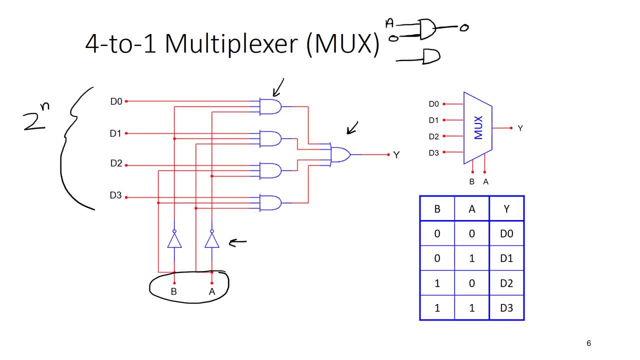 Here's another AND gate. This time I'm going to send in a 1 to this AND gate. Now I have a switch called A, So I'm ANDing together A with a 1.. That output is going to be whatever A is. 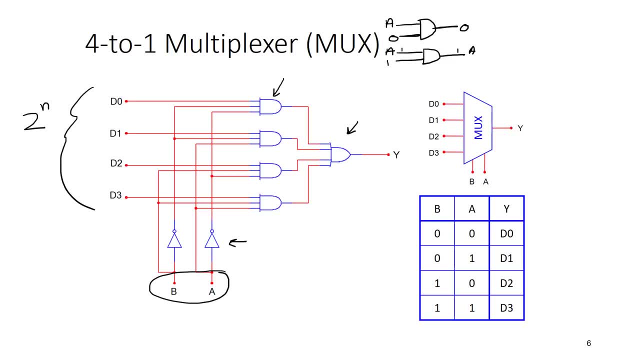 In other words, if I switch A on, I'll get a 1 out. If I switch A to a 0, I'll get a 0 out. So, effectively, if I make all the other inputs to an AND gate 1s. 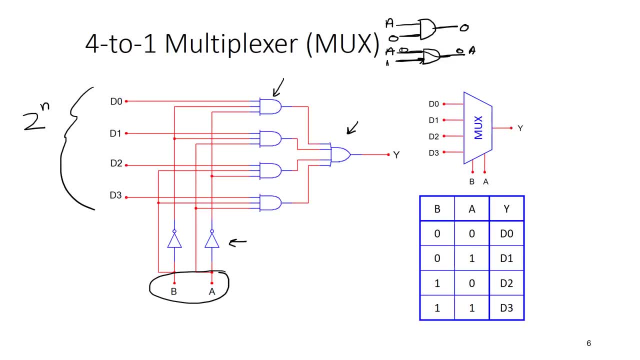 the output will be 0.. That's going to be whatever data is coming in on line A. That's the basis for how these things work. In other words, if I want D0 to be transmitted to my output, I have got to make sure that all the other inputs 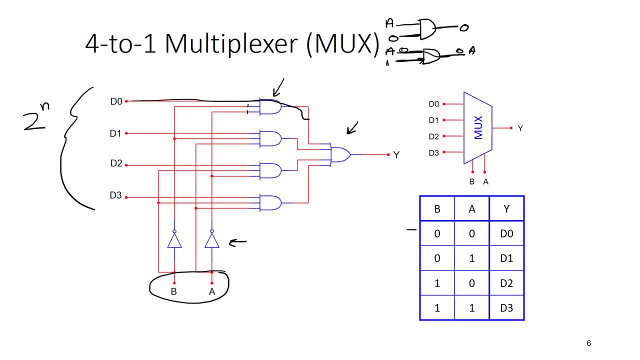 both these inputs are 1s. Well, how am I going to do that? Let's look at the table right here. It says: if I make A and B both 0s, my output will be D0.. Let's see why. 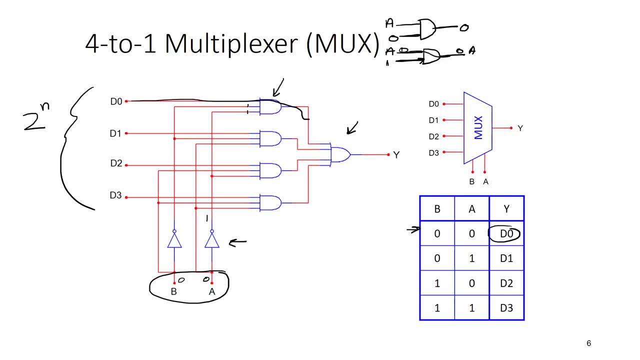 If I make these both 0s, them right here, so that means they're going to be 1s. I'll have a 1 going into both of these things, And so yes, in fact, whatever D0 is will be my output. And if we take a quick look at the 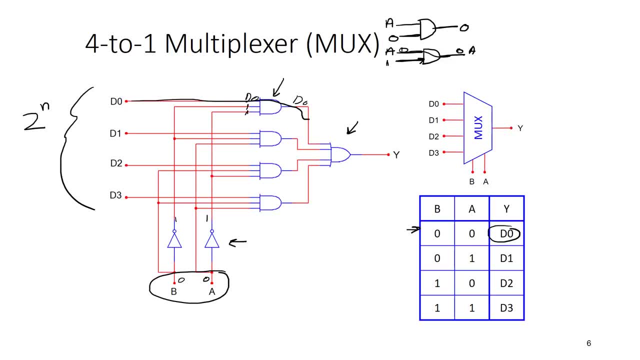 other, AND gates at the same time. let's see, remember I have zeros going in, so these two lines will be 0.. Let's just check out the other ones real quick. So this would be a 1, 0. This. 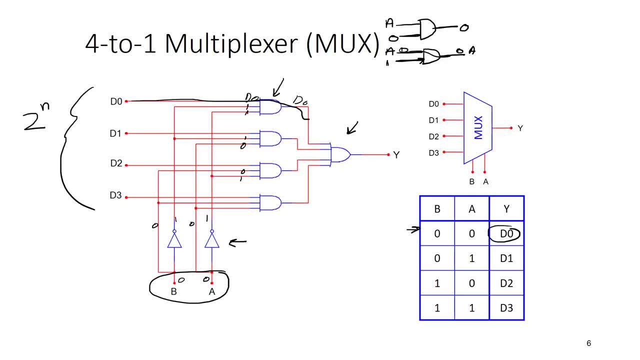 would be a 0, 1.. And this would be a. it looks like I have a 0, 0.. Yeah, So notice, when the inputs are 0, 0, the only AND gate that's enabled, the only one that has two 1s, is this top one. 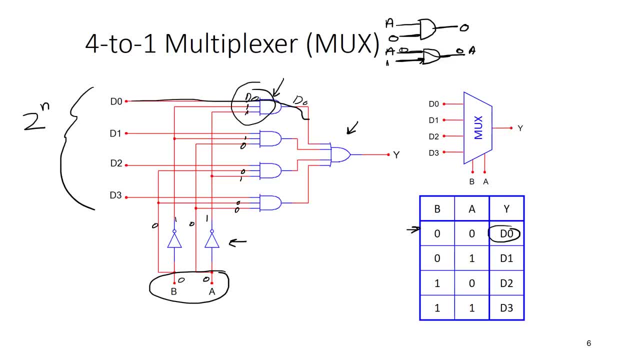 right here And I think if you follow the other examples- like if I wanted to check out what happens when B is a 0 and A is a 1, I think you will find that D1 will get two 1s and the output will come from this AND gate It's. 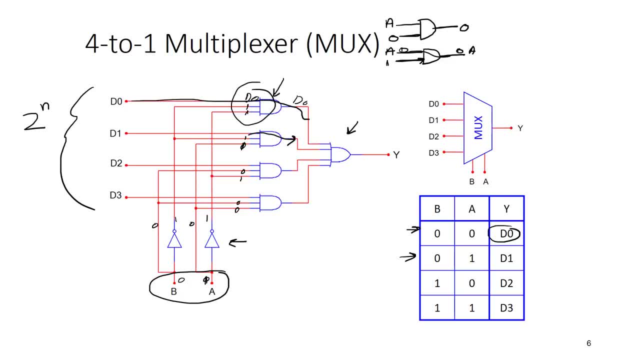 really not that complicated, but hopefully you get what's going on here. So again, a multiplexer just built out of basic ANDs and OR gates, and it's always going to be some power of 2.. In this case, I have four inputs and I need two digits to select which of the inputs goes to the output. 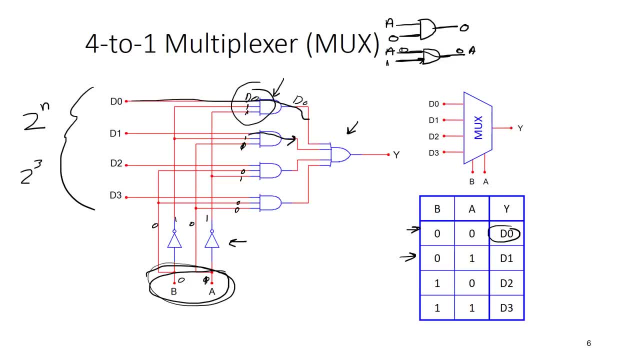 Let's say I had two to the third or eight inputs. How many different inputs would I need on the bottom to select which one went to the output? Well, it would be three. Why would I need three? Well, because in binary you need three bits to get eight possible combinations from 0, 0, 0 to 1,. 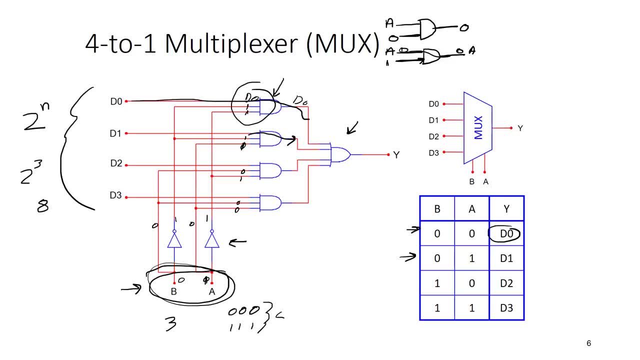 1, 1.. That's zero to seven, That's eight possible combinations. I would need three inputs on the bottom for my selectors if I had eight data inputs And, of course, if I had 16 data inputs I would need four different selectors: A, B, C and D. perhaps on the 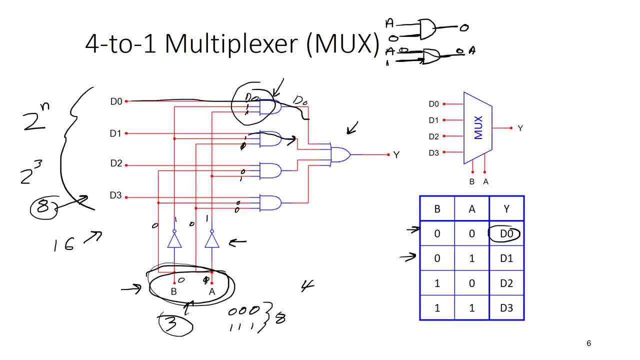 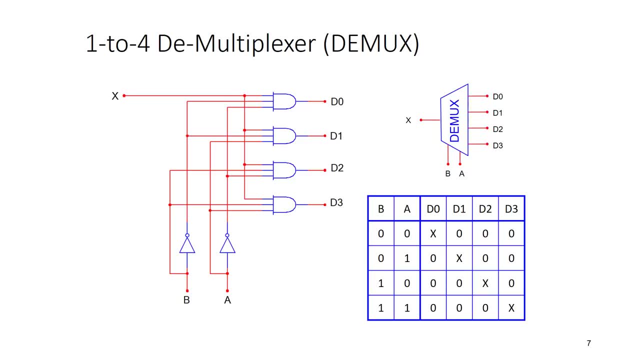 bottom. Hopefully this makes sense. Now let's take a look at D multiplexers. So here is what the inside of a D multiplexer looks like And amazingly, it is also made out of basic ANDs. So here are a bunch of three input AND gates. Here's a couple of NOT gates or inverter gates. 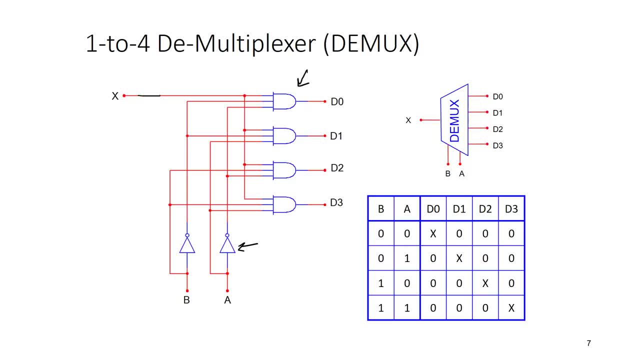 And let's see how this works. Remember a D multiplexer. I have my one input source and I can decide where I'm going to send that input, which one of these four outputs, And, of course, as you guessed it, the number of outputs is always going to be a power of two. 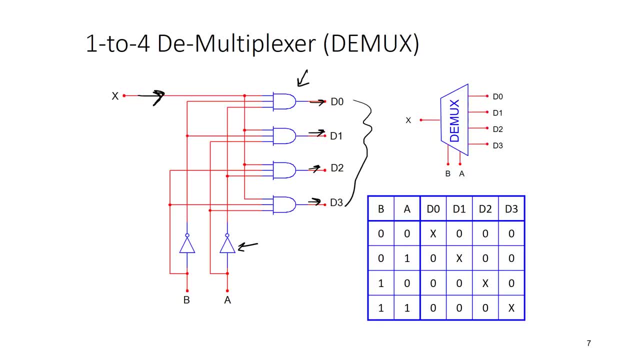 It's going to be two to the, something two to the N, two, four, eight, 16,, 32, and so forth, And the number of inputs is N. Well, we'll go over that. So let's say that I want. 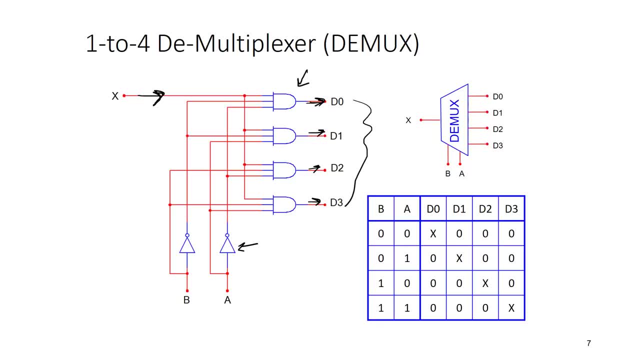 my output to go to D zero. Well, as you already know, if you want to transmit whatever the input is, I've got to make the other inputs both ones. Well, how am I going to do that? Let's look at this table right here. If I make them both zeros, let's do that. I'll make A and B both zeros. So if 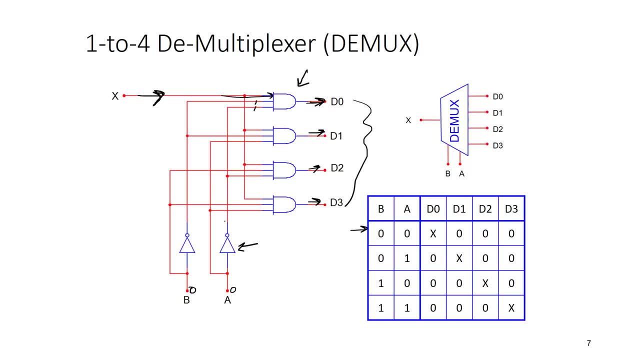 I make the output, A is a zero. Coming out of here, I will have a one and one, And going into here, yes, I have two ones. So my input coming from X will be transmitted to D- zero if I make them both. 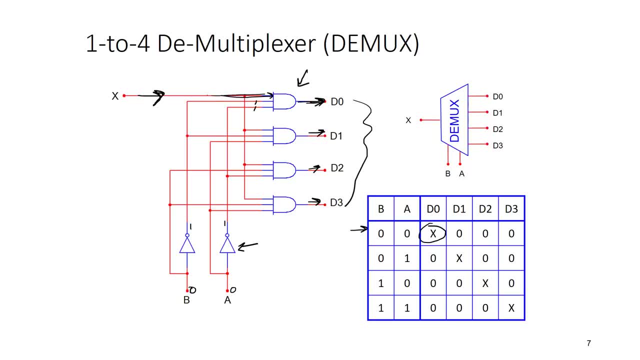 zeros. So yes, the output will be D zero. The others will be just zeros. If I want my data to come out of D one or to be sent to D one, I make A and B both zeros. So if I want my input to go, 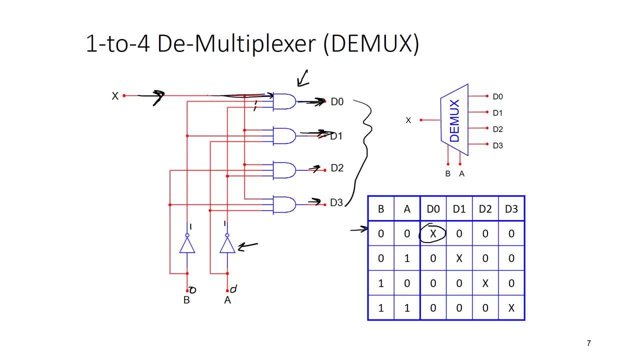 to D zero, I'll make A and B, both zeros. So if I want my input to come out of D one or to be sent to D one, I'll make B a zero and A a one And you can follow through this. This is very similar. 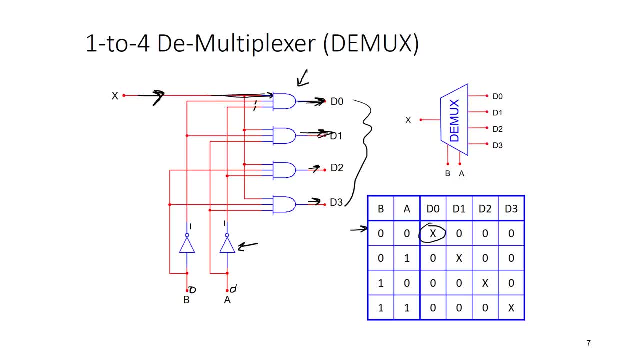 to the multiplexer diagram. The whole idea is: if you want to enable an AND gate, you've got to send all of the other inputs, ones, And then this last input, in this case, will be coming from X. Whatever X is will be transmitted to your output. And again over here this is the diagram of a. 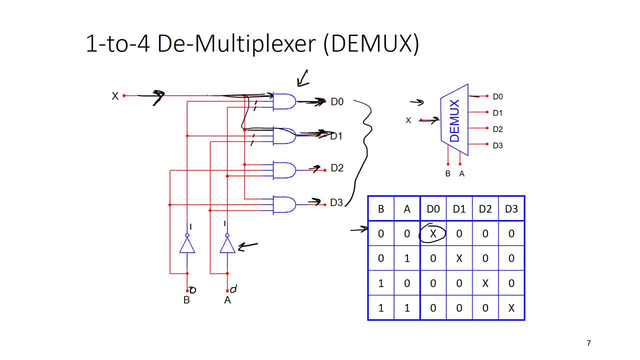 D multiplexer, one input, multiple outputs, And you can select one of the inputs And you can where your input gets sent by using these selectors on the bottom. And if I have, let's say, for example, let's say I have, 16 outputs, also known as two to the fourth, I will need four. 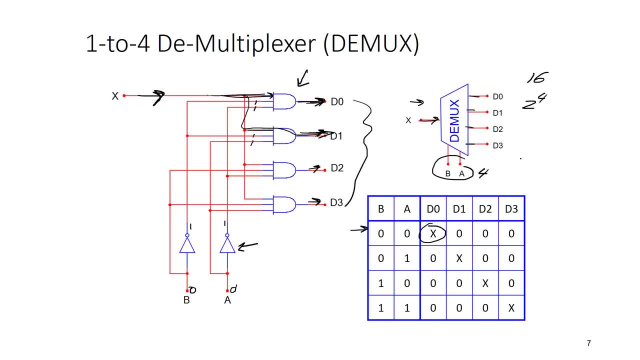 different input selectors. right, Because to get 16 possible numbers in binary I need four bits. I need to go from zero, zero, zero, zero to one, one, one one, That's from zero to 15, that's 16 possible combinations, All right. Well, hopefully that makes sense. A couple more. 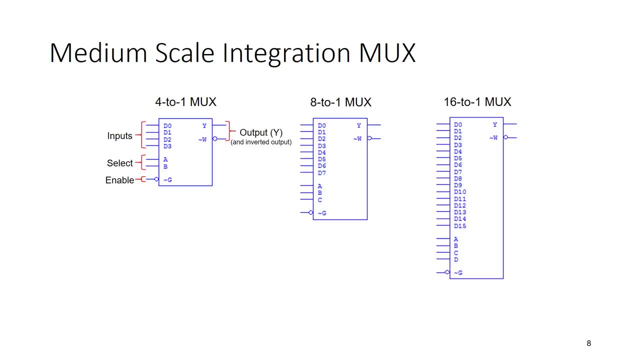 slides to go. So here's a look at what a multiplexer will look like if you work in multisim, And here's a bunch of different multiplexer chips. Here's a four-input multiplexer. right, I have four inputs And you can see that I will need two switches to select. 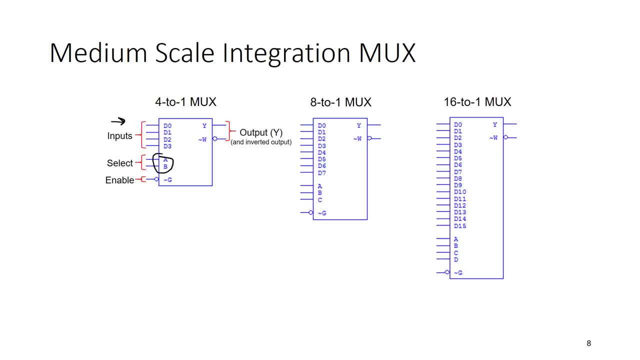 which of these four inputs I want. And here's an eight-input multiplexer. In this case, it's a four-input multiplexer. And here's a four-input multiplexer. And here's a three-input multiplexer. So I'm going to need three inputs. to select which of these inputs, 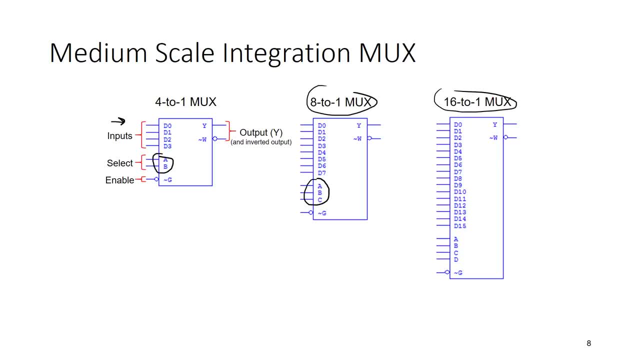 goes to my output And, of course, if I have a 16-input multiplexer, I'm going to need four switches. This other little pin here, this is an enable pin, And notice it has a little bubble, a little circle right there. That circle means in order to enable this particular chip. 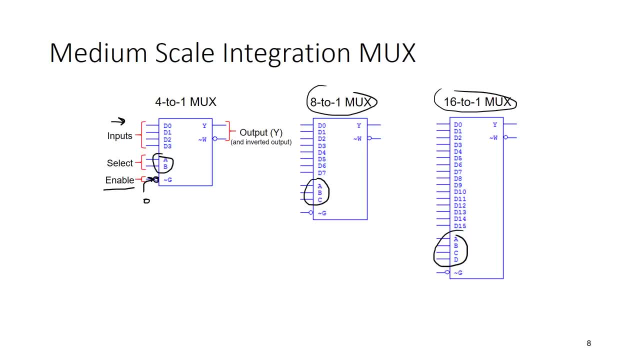 you need to send it a zero. That little circle indicates that it wants a zero to do its job. So another way of saying it is: it's active low. You will activate this chip if you send it a zero. Notice that all the chips have that little enable right there. So in order. 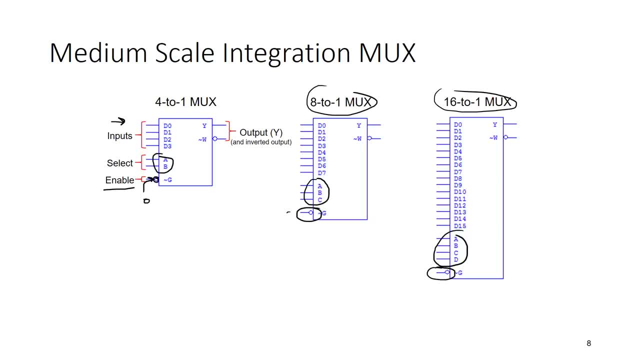 for this chip to work properly- and I don't know why they designed it this way- in addition to your inputs and selectors and all that kind of stuff, you have to send this little activation pin a zero. All right, let's take a look at demultiplexers. Finally, let's take a look at the. 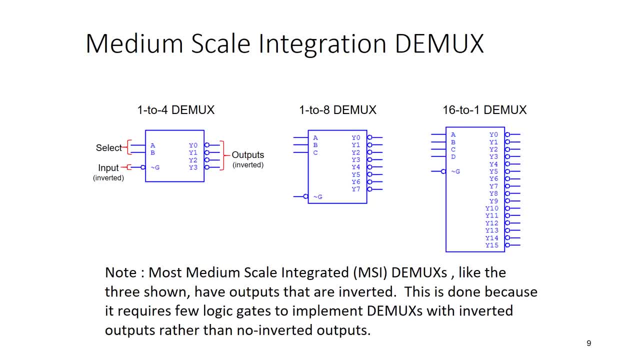 diagrams of demultiplexers. So this is what it's going to look like in multisim if you work with demultiplexers. Here I have a four-output demultiplexer And of course, I need two switches to determine which output it goes to. This is my input right here. Here I have 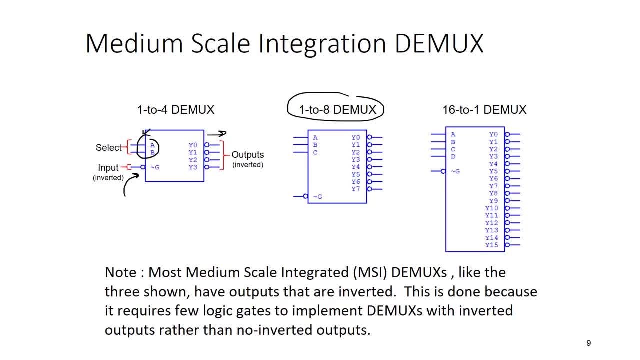 a 128 demultiplexer. Again, this is my data input line, And I need, of course, three switches to determine which of these eight outputs it goes to. Then I have my 1621 demultiplexer. I need four switches to determine where my data is going to. 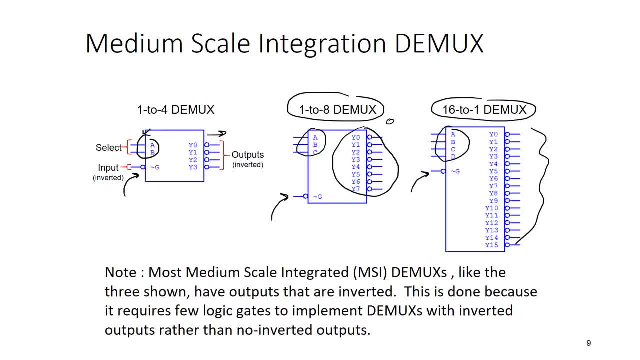 be sent from these 16, right Four switches. 0000 to 1111 is 15, or rather 16 possible combinations. I need 16 combinations to determine which of these 16 outputs it's going to go to, And notice also at the end: these little bubbles here mean that the output is going to be. 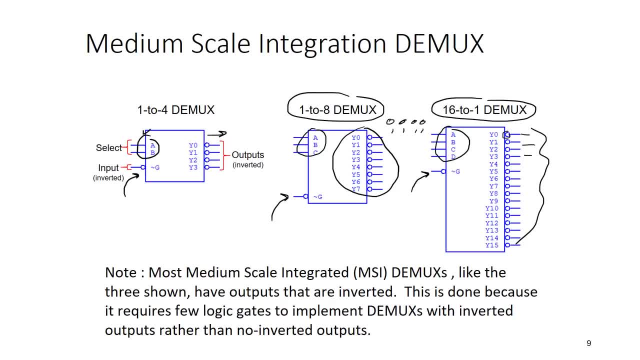 converted. It's done. I know that seems weird. Some chips are built like this And presumably it's because it made the logic inside the chip a little bit simpler. You really don't need to worry about that too much with multiplexers. We'll talk more about that when we talk about